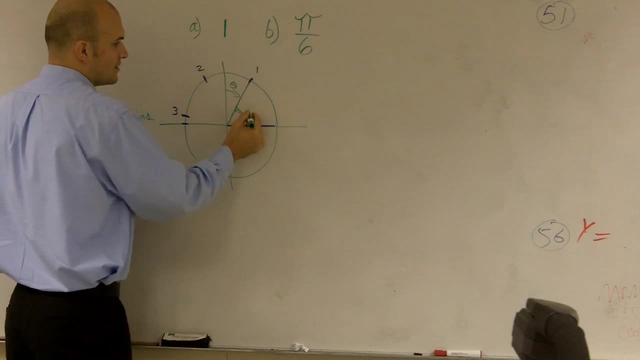 So to find the complement, we need to find this angle right there. So that's one radian. we need to figure out what that is And then remember our formula: To find the complement, we just do pi over two, which represented 90 degrees minus one. 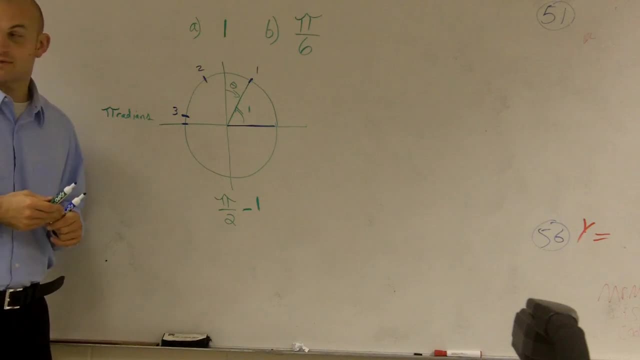 And then, after you look at this, you say: oh well, how do you do? How do you do? pi over two minus one. Well, one thing I can do is I can make these two the same fraction, So I can multiply by two over two. all right, 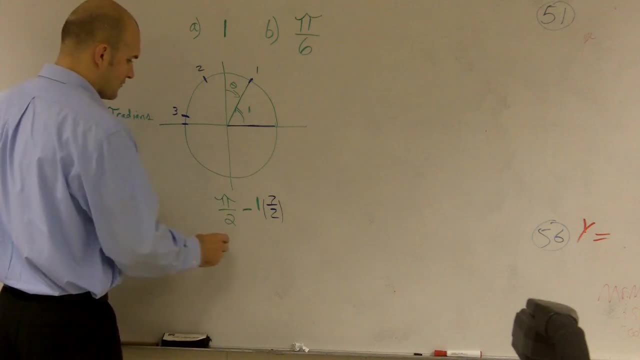 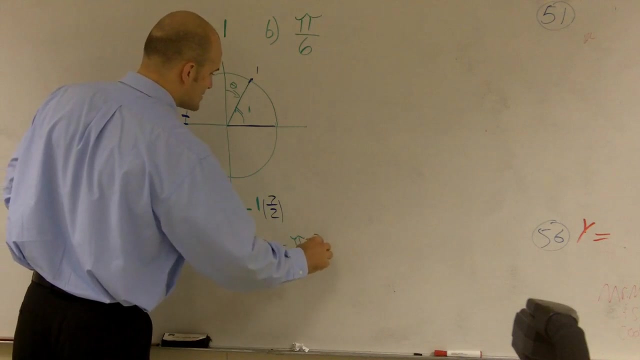 And I don't have a calculator to approximate this. But therefore you have pi over two minus two over two, which equals pi minus two divided by two. So if you have a calculator you can just do pi minus two divided by two, okay. 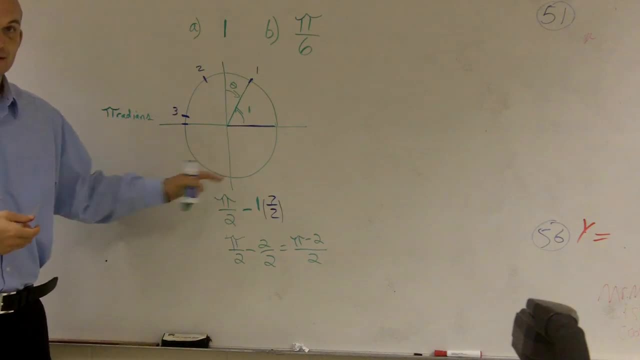 And that would be your answer. If I wanted to find the supplement and remember the supplement, the supplement is right over here. This is that pi. So if this was pi over two, if I want to find the supplement now, I'm looking for this angle from there to there, right? 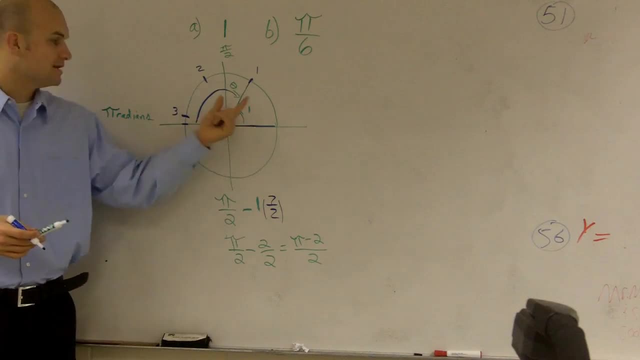 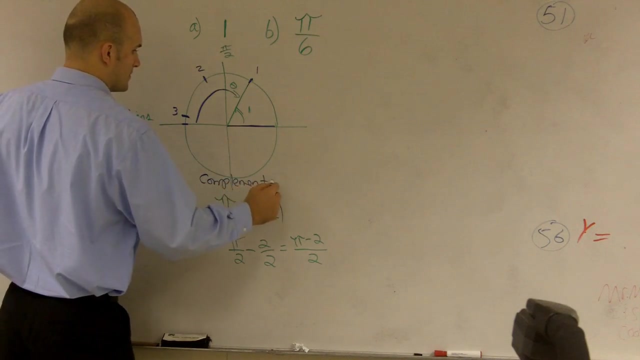 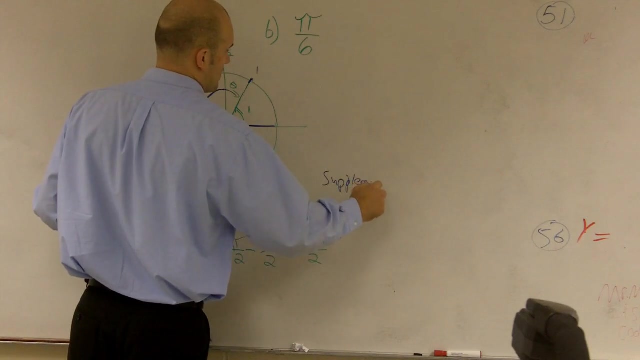 The supplement is what part of your angle will add to your one to get to 180.. So for the supplement, this is complement. So for the supplement, for the supplement, what I'll do is the same thing. I'll just do pi minus one. 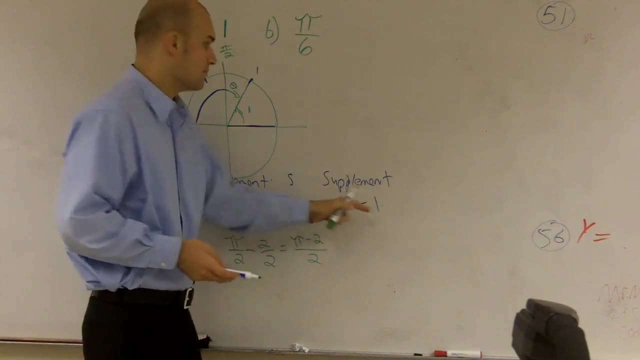 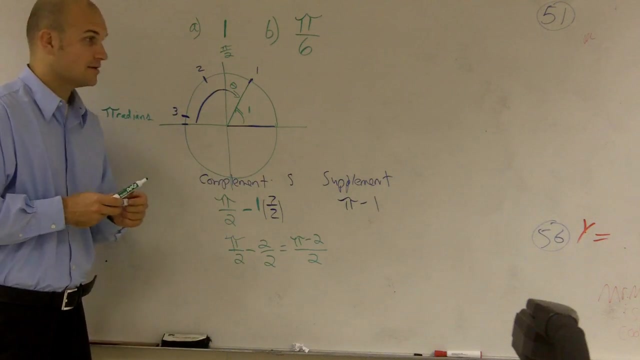 And, like I said, I don't have a calculator with me, but you guys can just take pi minus one and that will give your angle for that. Does that make sense? Okay, But now see, the difference is. that's just dealing with where you're at. 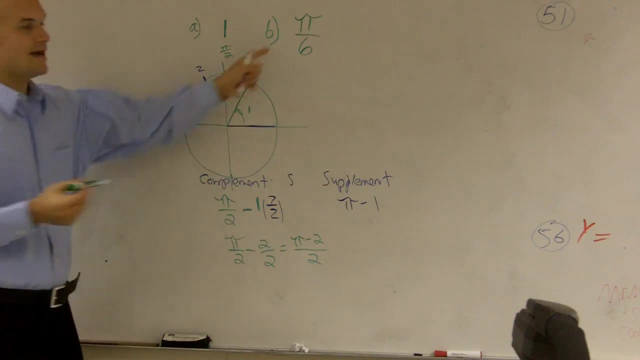 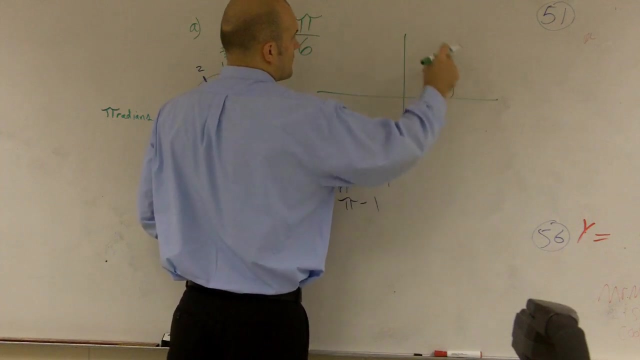 So you just always have radians. It's just your radius wrapped around it. But when I have something like pi over six, that's a little bit different. All right, Because we know that here is pi, right? Did I get you to believe that that's over? there is pi. 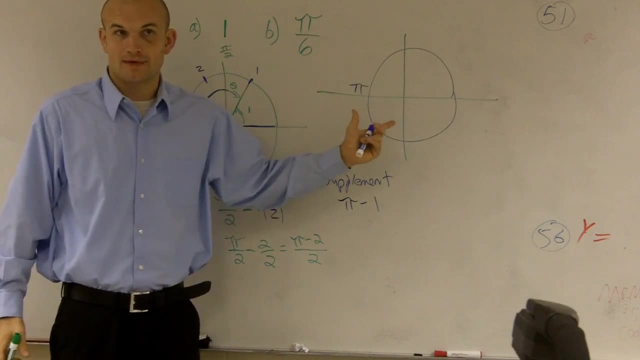 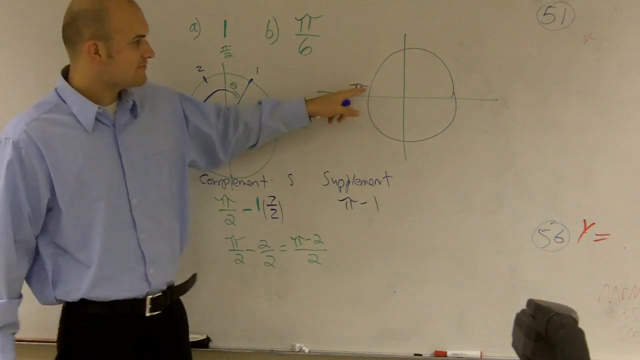 From here to here is pi radians. Okay, It's pi radians, It's not one, It's not two, It's not three, It's pi radians. So since from here to here is pi radians, I want to say what is one-sixth of that?